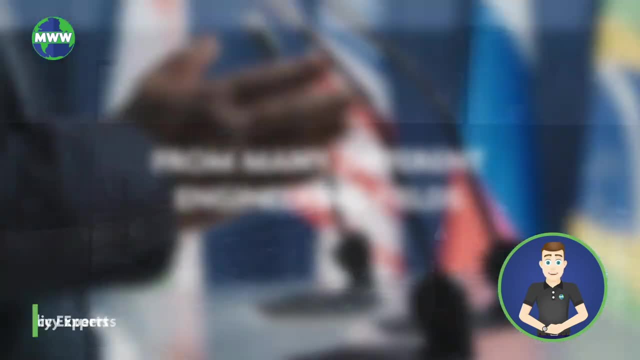 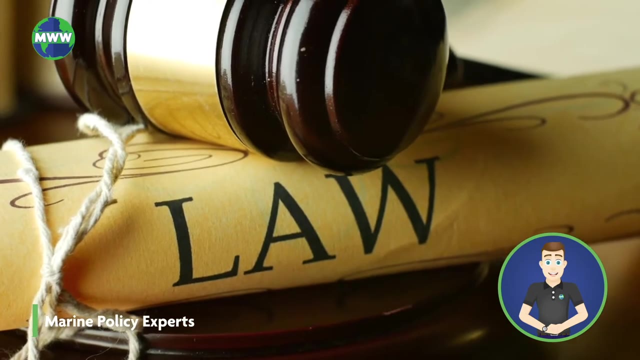 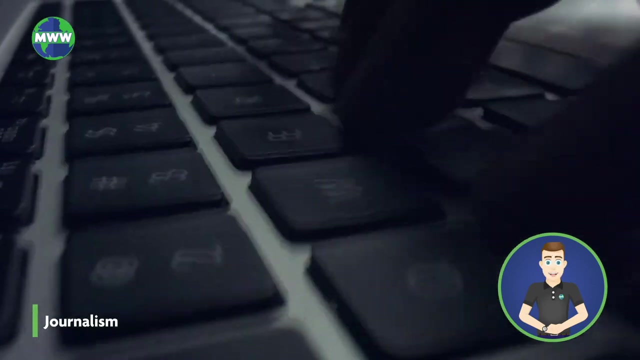 mechanical, civil and chemical engineering. Marine policy experts combine their knowledge of the ocean sciences with the social sciences, working to create policies, guidelines and regulations for the use of ocean and coastal resources. Journalism allows for the spread of important information about oceanography to the general public. 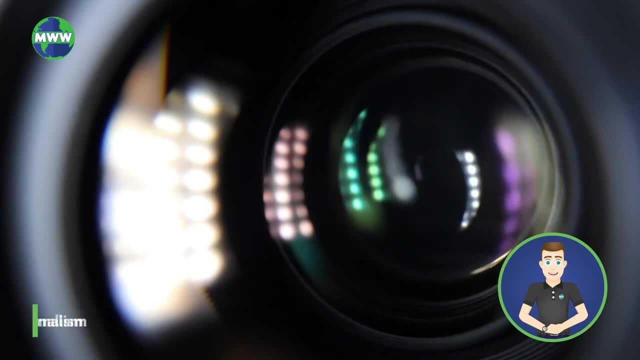 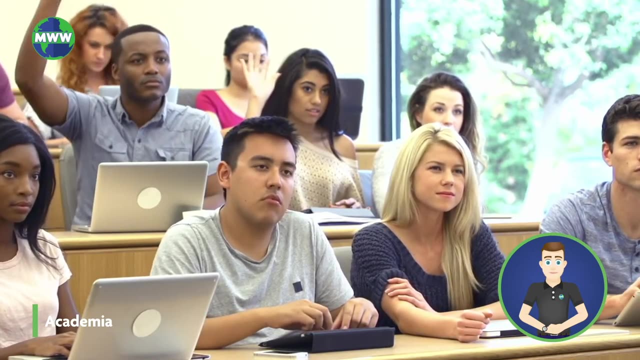 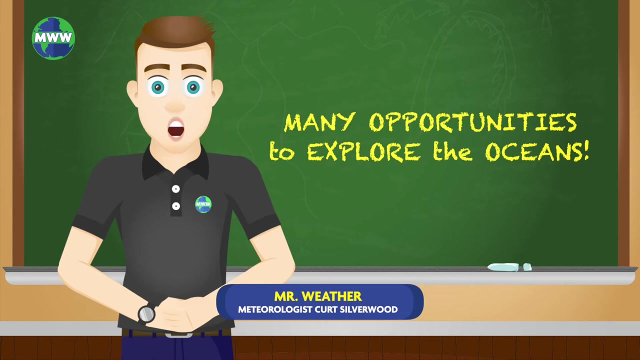 They can work for newspapers, magazines or television and radio. Those in academia range from middle and high school science teachers to university professors. At the university, professors are often part of research projects and other types of fieldwork. Overall, there are many opportunities for those who want to explore the oceans. 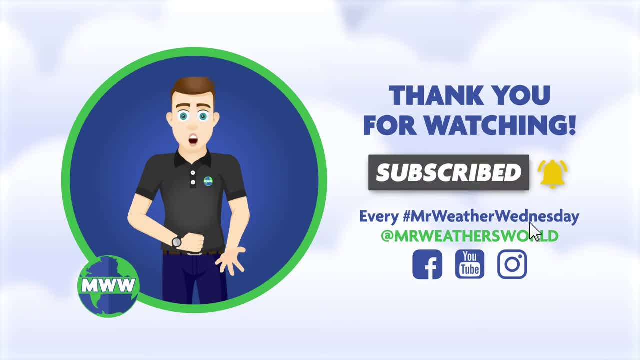 Thank you for watching. Please subscribe to Mr Weather's World on YouTube for new videos every Mr Weather Wednesday.